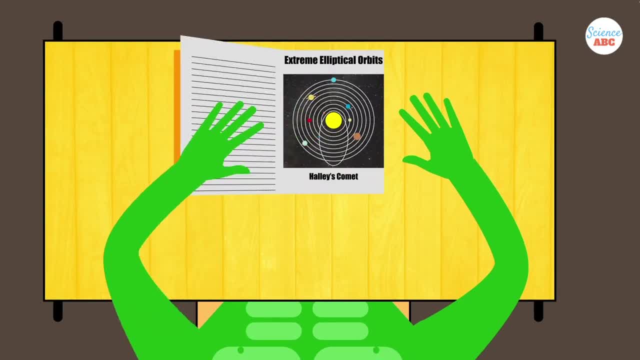 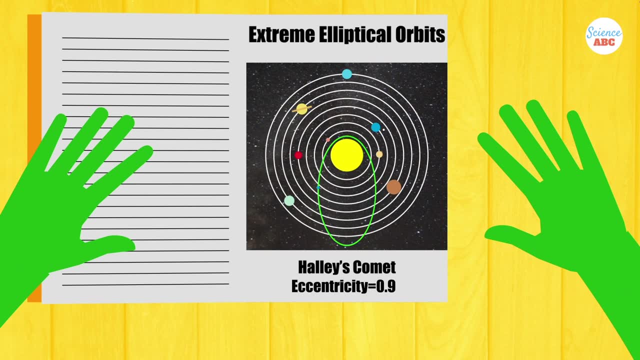 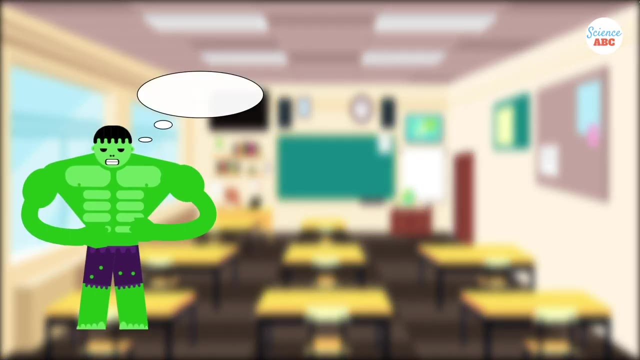 what an extreme ellipse could be. there's a great example to look at: Halley's Comet. Halley's Comet follows a path with an eccentricity of approximately 0.97.. Just look at how elongated its elliptical path is. But the question still remains: why aren't the planetary orbits? 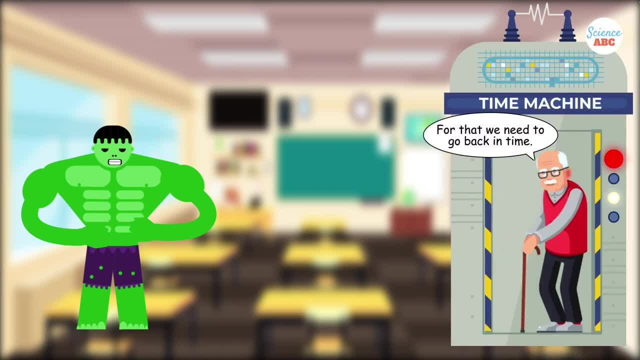 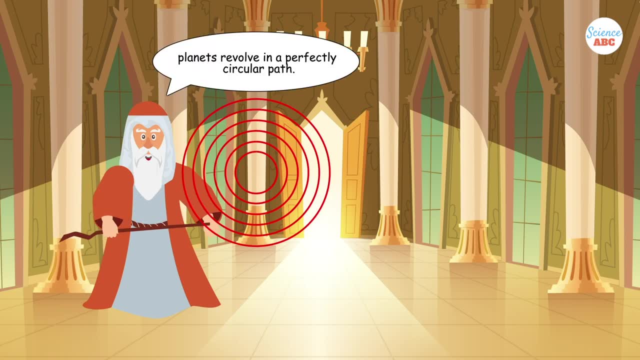 perfectly circular? Well, for that answer we need to go back in history. For a long time, from Ptolemy to the age of Copernicus, it was widely believed and accepted that planets revolved in a perfectly circular path. This was until Kepler came along and laid down 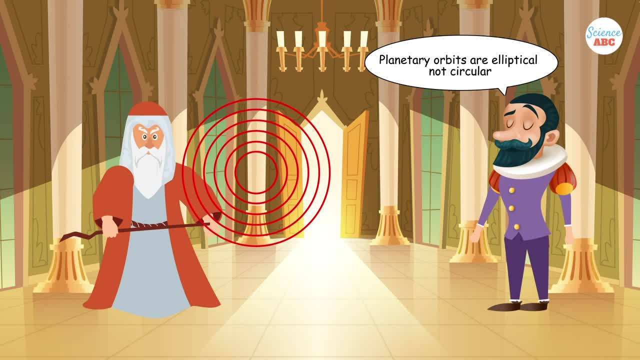 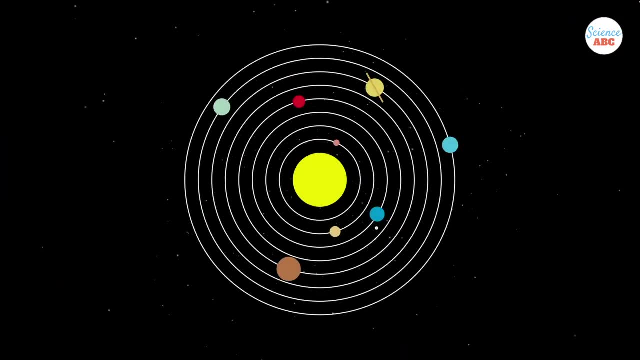 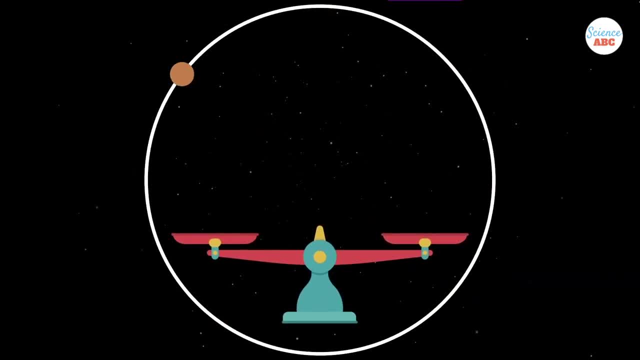 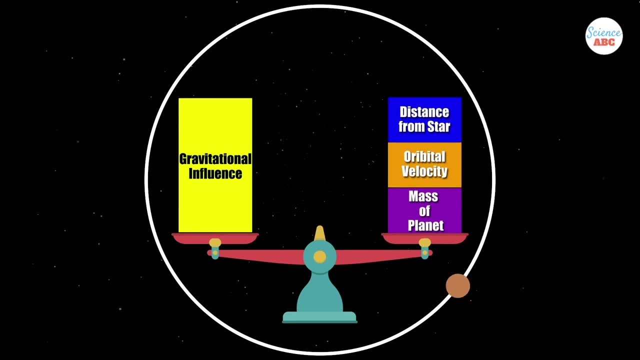 a perfectly circular orbit, the orbiting planet would need to have mass velocity and distance from the star that precisely matches the gravitational influence of that star. A slight change in any of these variables would derail the planet from maintaining a perfectly circular path. 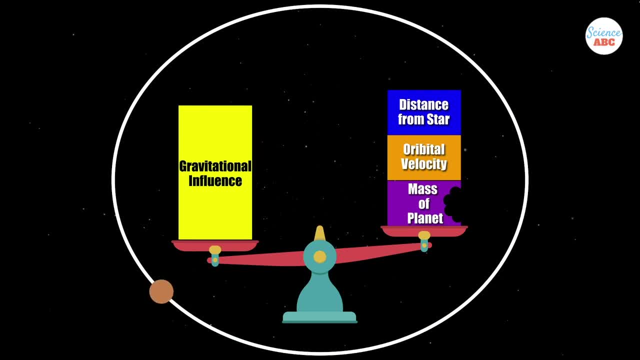 For example, if the mass of a star or planet changes, or any other celestial body whizzes past that planet, it would disturb this delicate balance of mass, velocity and distance That's that keeps a planet in a circular orbit, and it would therefore change it to an elliptical one. 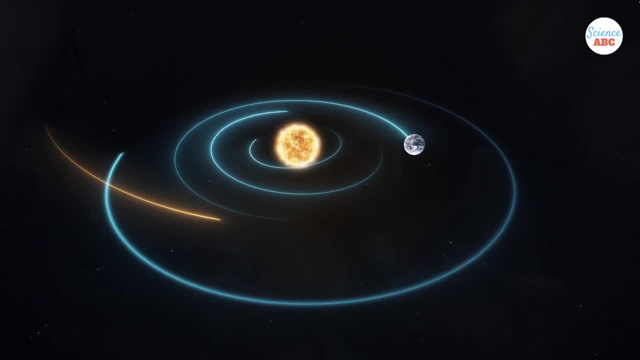 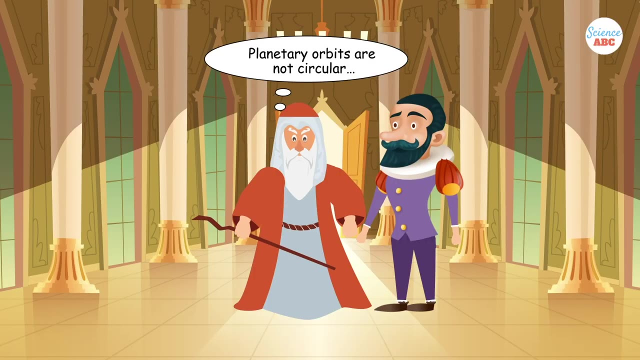 Even a small tweak in these status quo conditions or any interplanetary interactions would change the path from a perfect circle. Despite fretting about orbits being not perfectly circular, it is worth understanding that these orbits are still closer to being circular than they are to 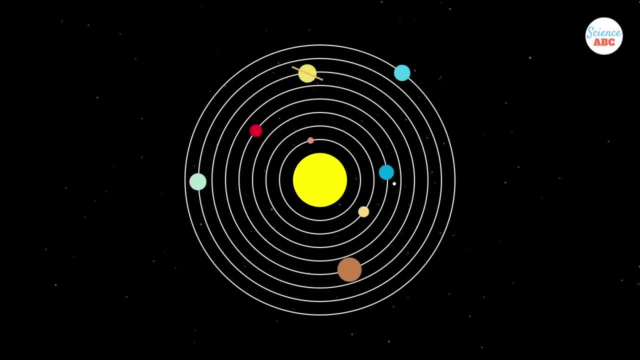 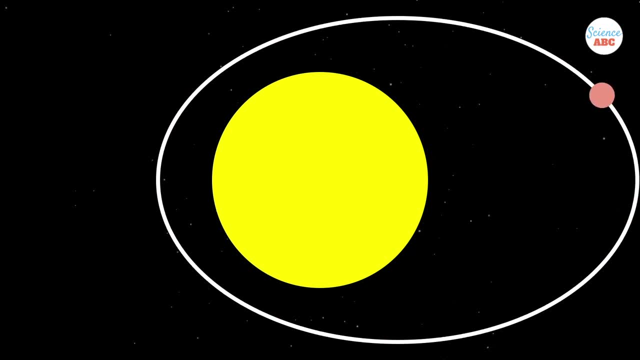 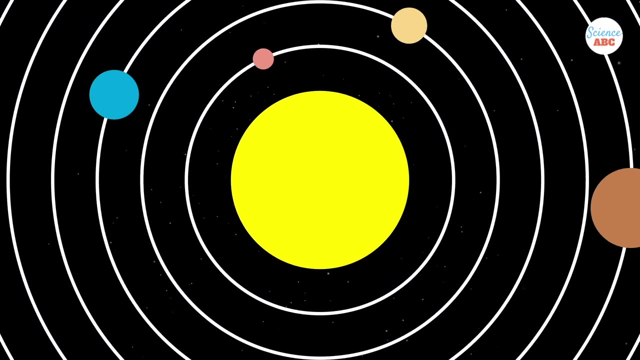 being highly elliptical, which is perhaps why the planets we see today have survived the test of time. Planets with highly elliptical orbits are more likely to run into trouble as compared to a circular counterpart. Why is that? Well, think about it like this: The planetary model taught: